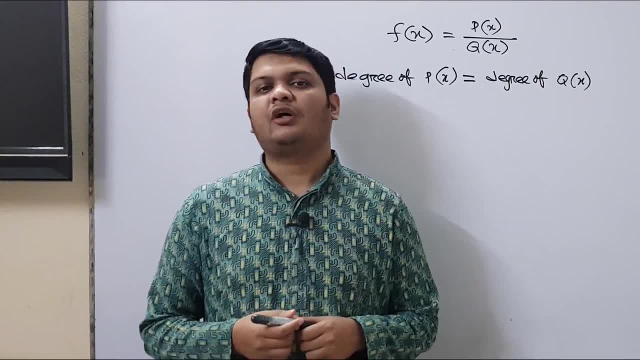 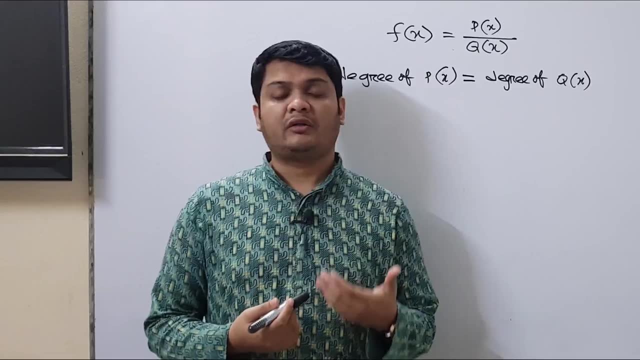 Assalamualaikum, I'm Pavel and I welcome you all to the sixth video of the calculus video tutorial series. In this video, we will learn about infinite limit and rational function. In the previous video, we already learned something about the application of infinite limits in rational functions. In this, 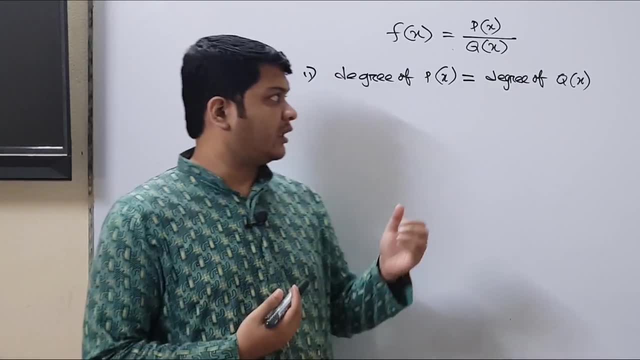 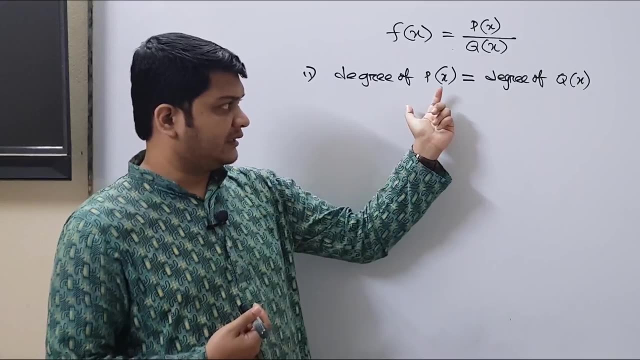 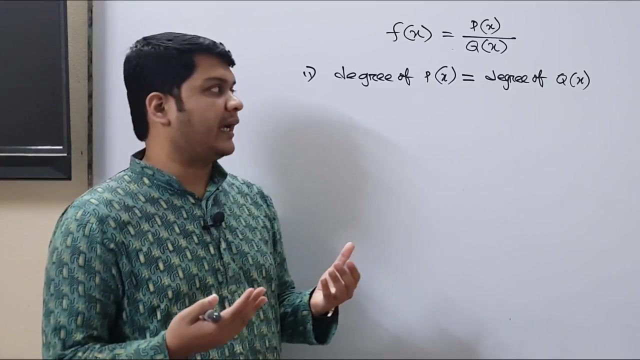 video we will discuss about case 2.. That is, you can see on the screen that whenever in a rational function the degree of p of x is equal to the degree of q of x, That is, the degree in the numerator and the degree in the denominator is equal. And in that particular case, what will be? 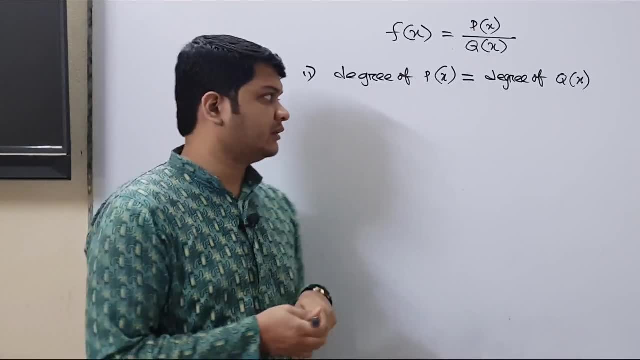 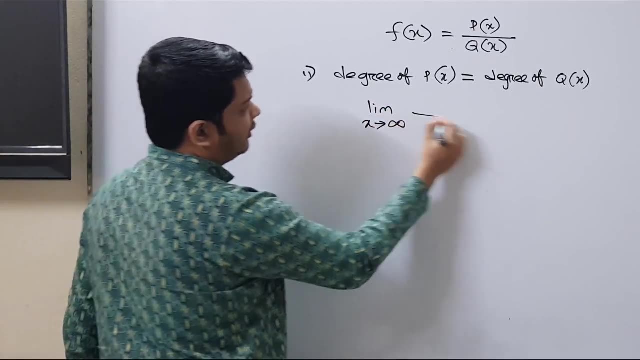 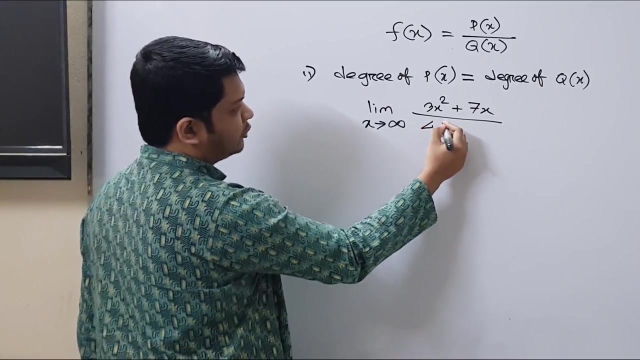 the outcome of infinite limit. So let's see some examples. Suppose we have a problem like this: Limit x tends to infinity, 3x square plus 7x, and in the numerator we have 4x square minus 5x. Suppose we have this problem. So, as you can see, this is infinite limit. 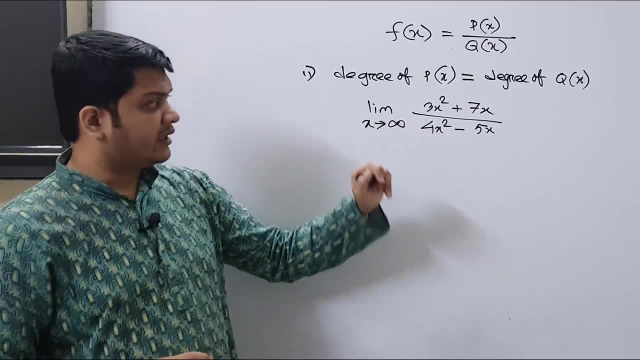 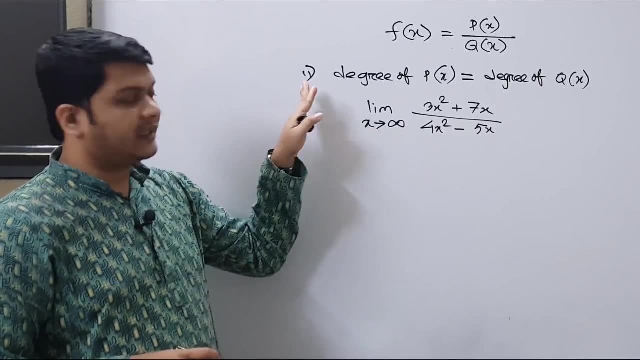 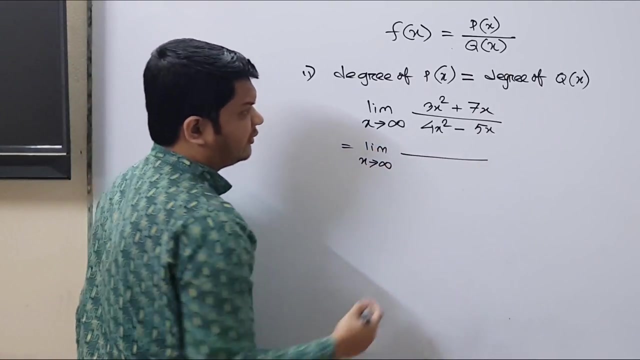 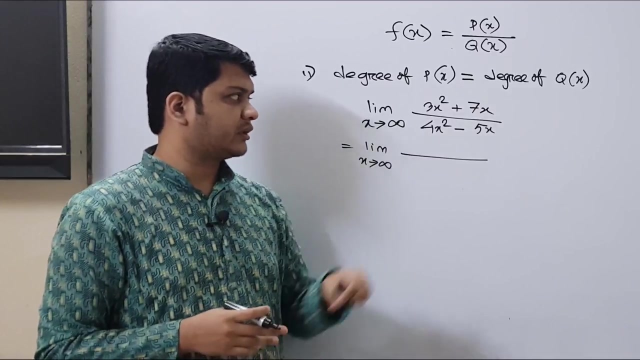 That is, x tends to positive infinity and the degree in the numerator is 2 and degree in the denominator is also 2.. So we are in case 2. That is, the degree are equal. So what we do do here is that, if you already watched the previous video, we know that we need to divide both the terms. 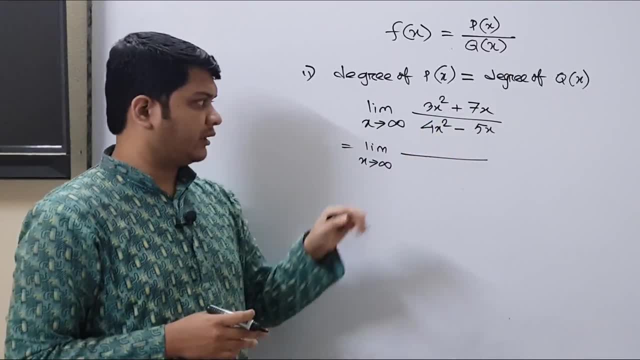 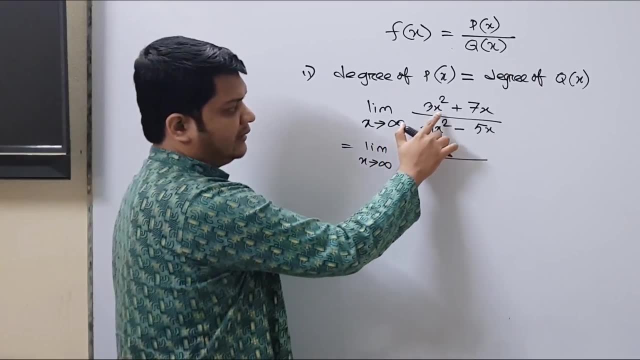 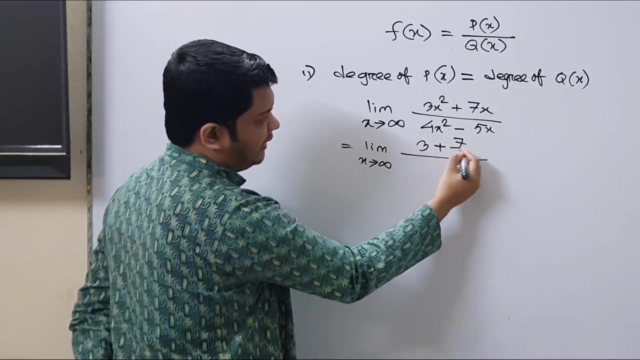 in the numerator and in the denominator. So here we will divide all the terms with the maximum power that we have here as x square. So we will divide 3x square with x square, So we will get 3 plus 7 divided by x. and if you divide 4x square, you get 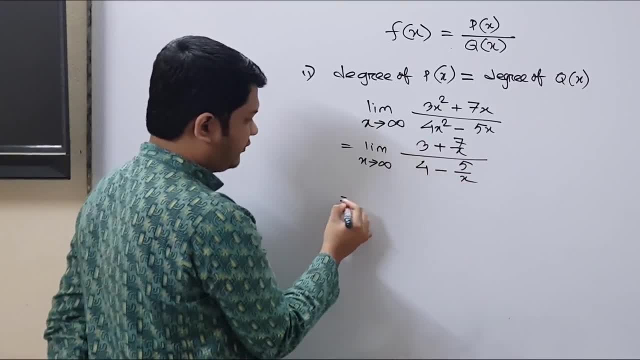 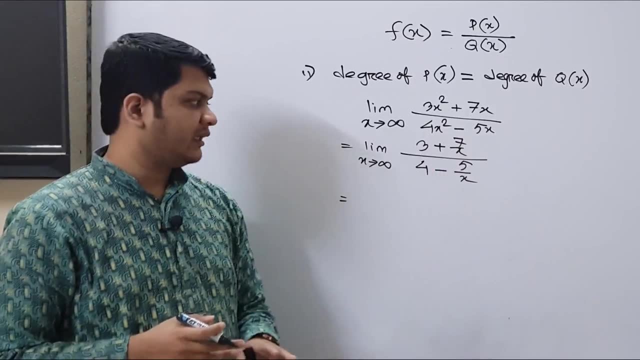 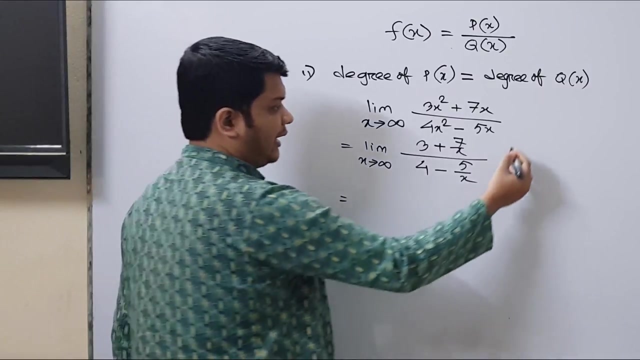 4 minus 5 divided by x. So we will end up here. Now the rest of the part is quite easy. This is exactly similar to the concept that we learned In the previous video, that is, we will apply the variable value here. that is, we will apply this. 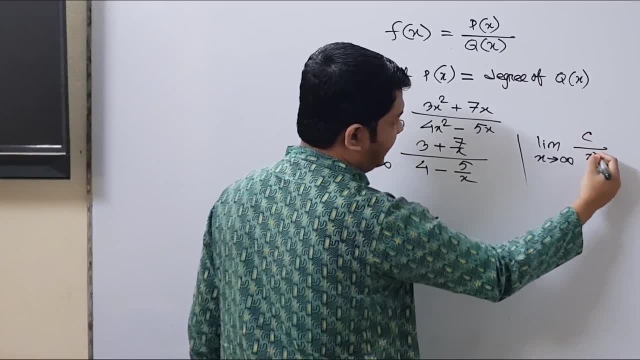 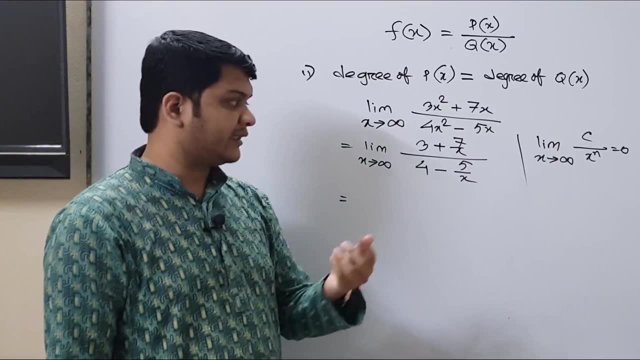 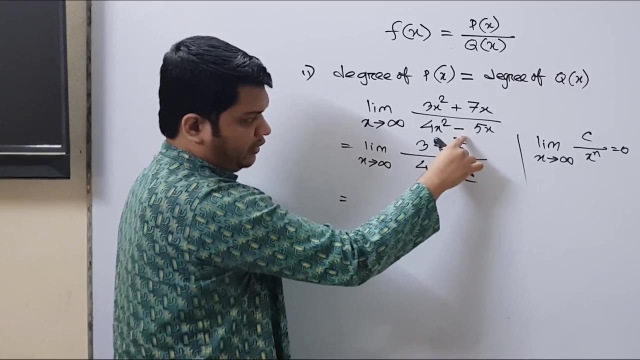 concept for limit x tends to positive infinity. c divided by x to the power n, this is equal to 0.. I already discussed this concept in the fourth tutorial So you can watch that if you still have some confusions. So, using this concept, we will get the value of this part as 0.. Also, we will 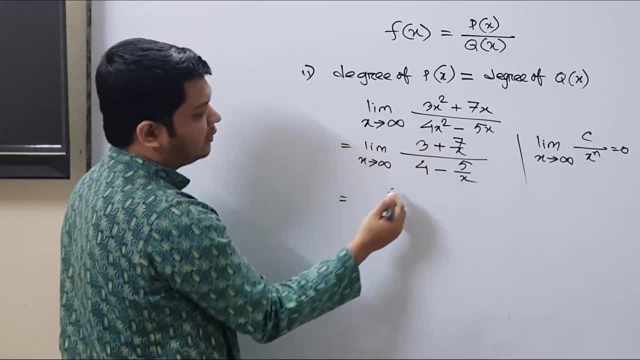 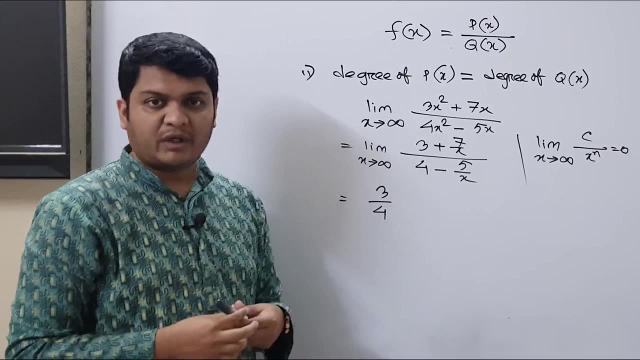 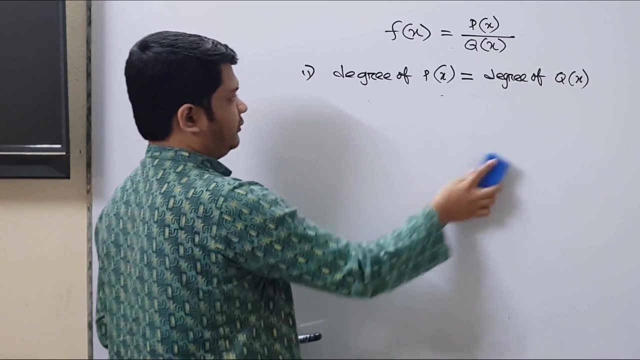 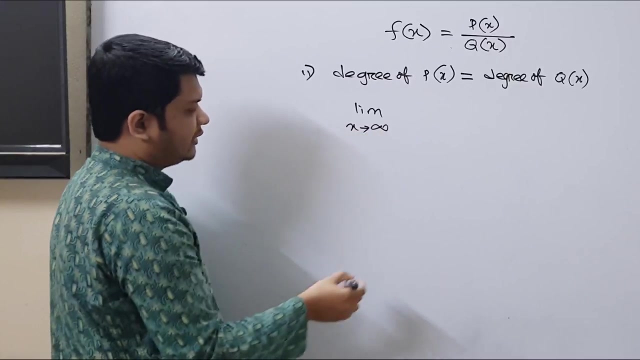 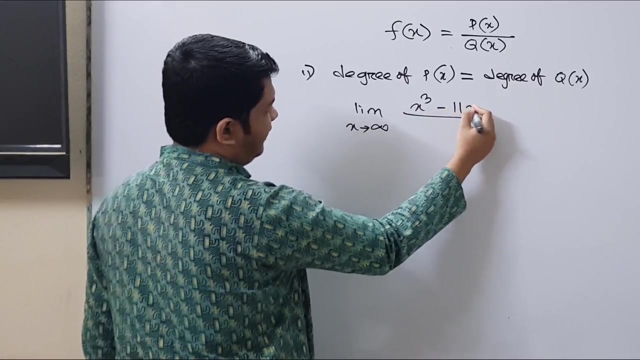 get the value of this part equal to 0.. will end up with 3 divided by 4.. I hope you understood it Now. let's solve few more examples so that you have a better and clearer idea. Let's solve another example. Limit x tends to infinity. Suppose we have x cube minus 11 x divided by 3 x. 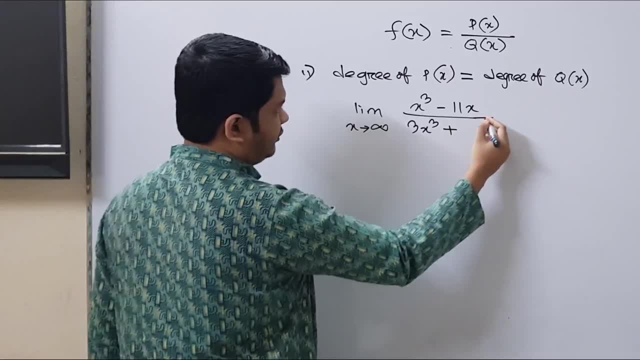 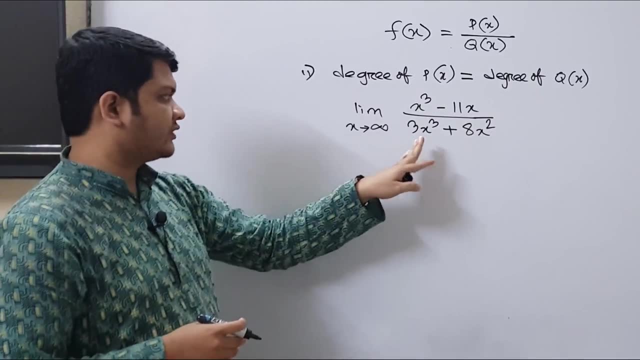 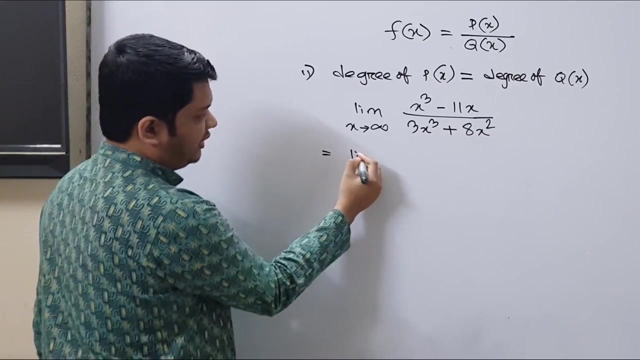 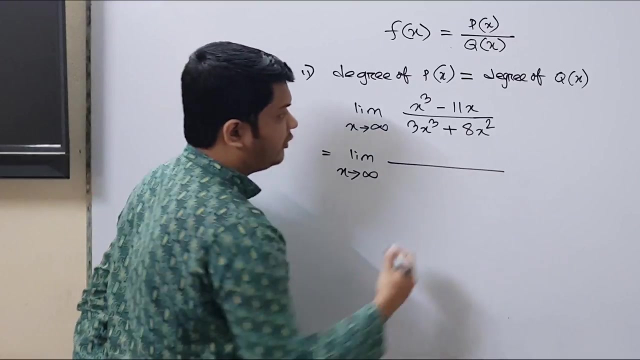 cube plus 8 x square, Suppose we have something like this: So here also you can see that the degree in the numerator and the degree in the denominator is equal. So we will now calculate rest of the part. So for limit x tends to infinity, we will. 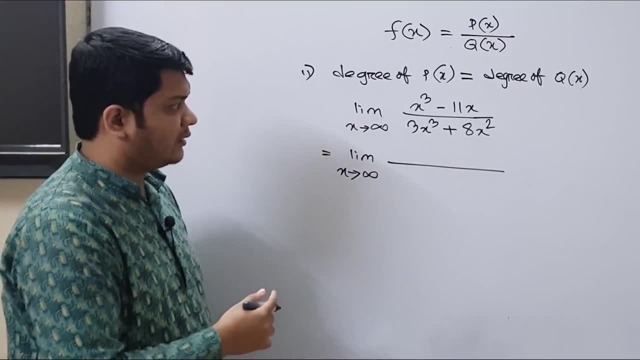 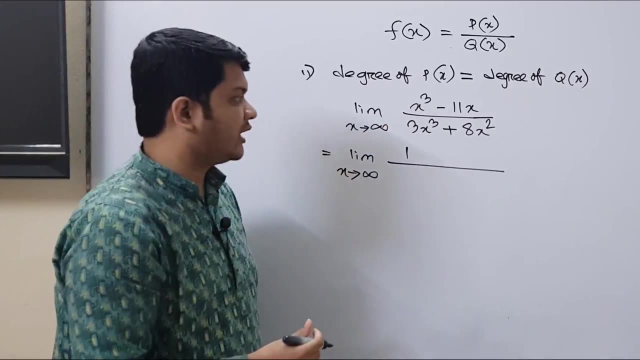 apply the same concept like the previous one, So we will divide all the terms with the maximum power, that is x cube. So we will get 1.. If we divide x cube with x cube, we get 1 minus 11, x divided by x cube. so we will get 11 divided by x. 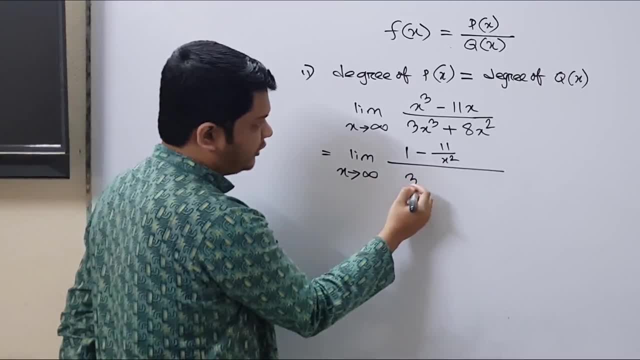 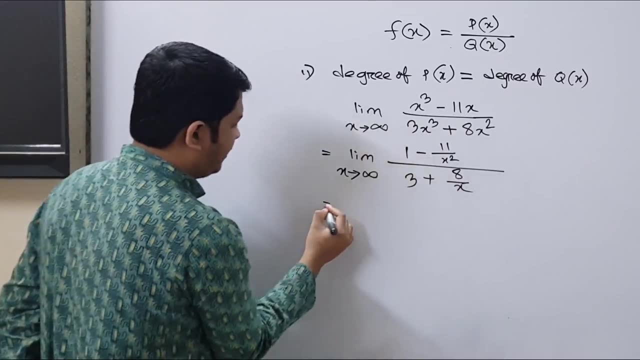 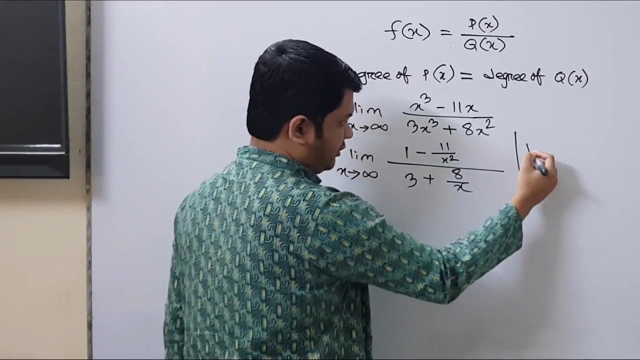 square Here: 3 x cube divided by x cube, so we will get 3 plus. if you divide x, 8x squared with x cube, we will get 8 divided by x. now you can see that these two parts will be equal to 0, like the previous one. let me repeat: limit: x tends to infinity, so c divided by x to. 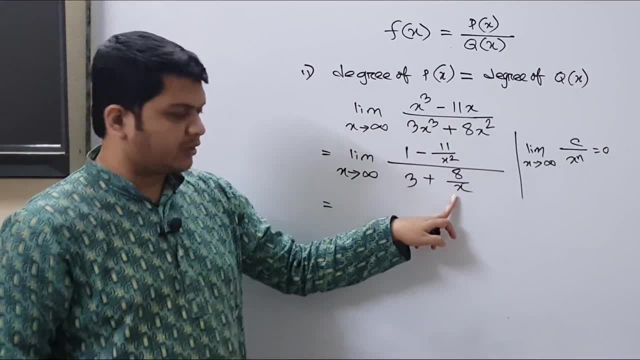 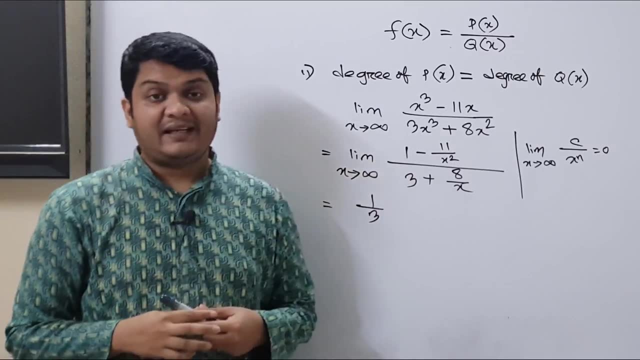 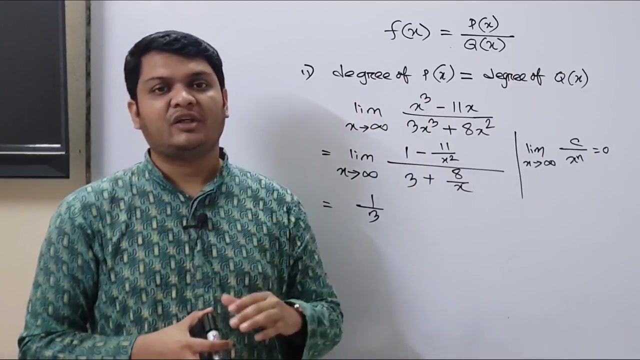 bar l is equal to 0, so this part will be 0, this part will also be 0, and we will end up with 1 divided by c. so this is the answer right now. i will show a trick here through which you can solve this type of problems very easily, within just one to two seconds. okay, let's see. so if we 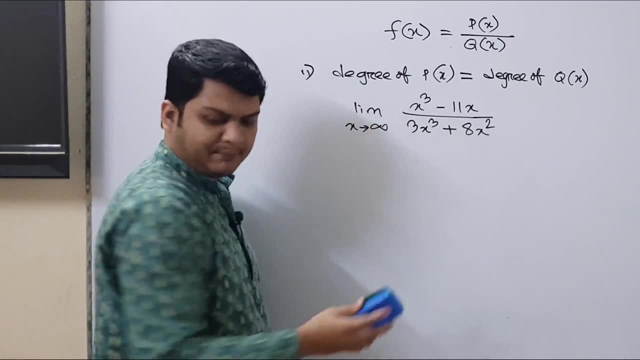 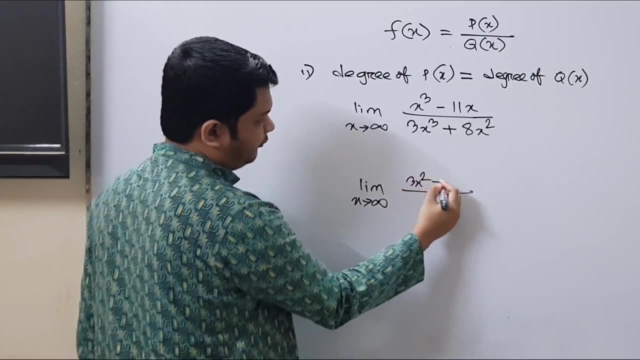 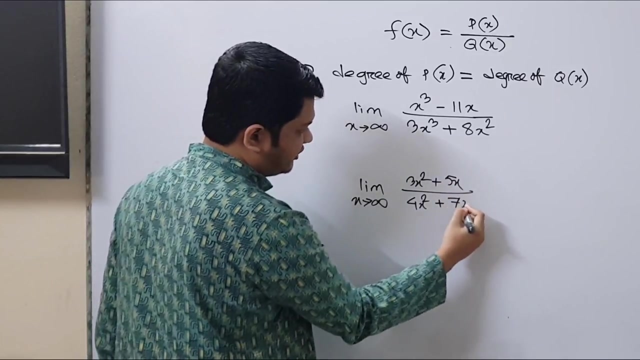 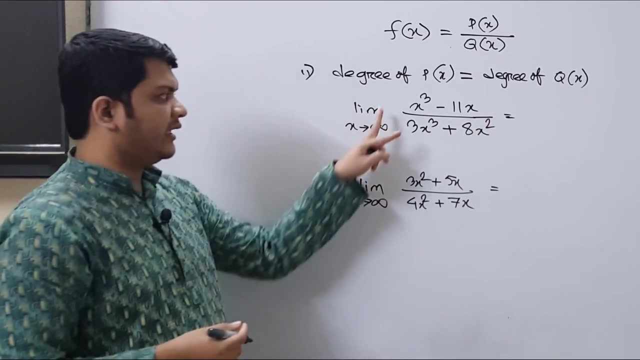 considered the previous example, it was something like this: limit x tends to infinity. we had 3x squared plus something x, and here we had 4x squared, so say, plus 5x or plus 7x. so this is the same as this concept, that is, the degree in the numerator.